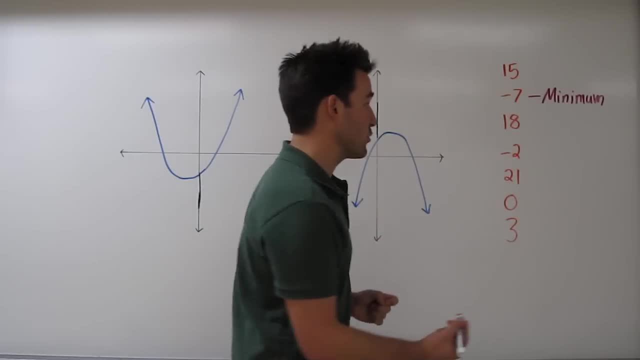 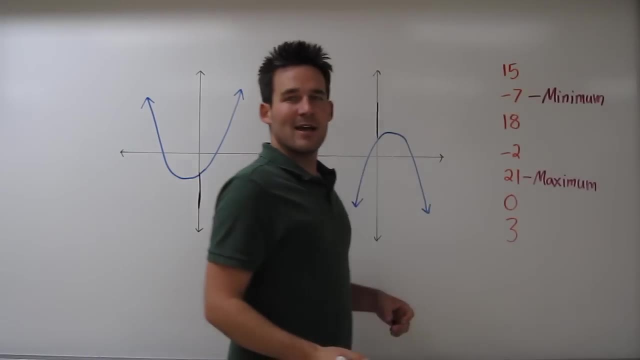 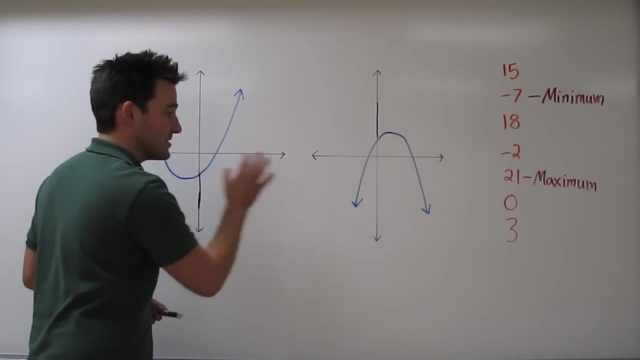 which looks like 21, is the greatest number, so we call that the maximum. Now we can also find the minimum and maximum of graphs of functions. Here we have two different parabolas graphed And by looking at this first one I see that the minimum value or the lowest value on the graph 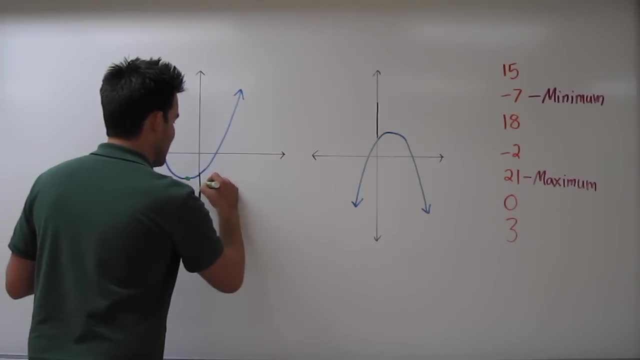 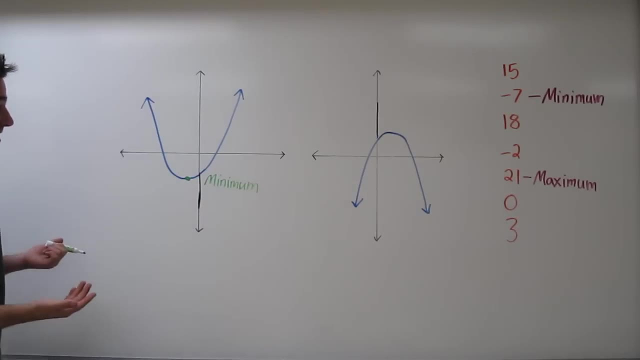 is negative 7.. The lowest value is right here, So let me write minimum. Now to find the maximum on this first graph it's actually kind of difficult. I mean, I see it's really tall up here, but I also know those arrows indicate that it keeps going up. 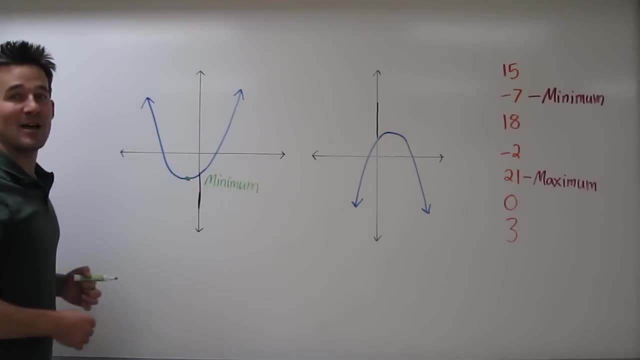 So actually this has no maximum. It just keeps going up and up and up. It's difficult for us to find the greatest number because it keeps going, But I am sure that this is the minimum. Now, if you remember some stuff about parabolas, this is also called the vertex. 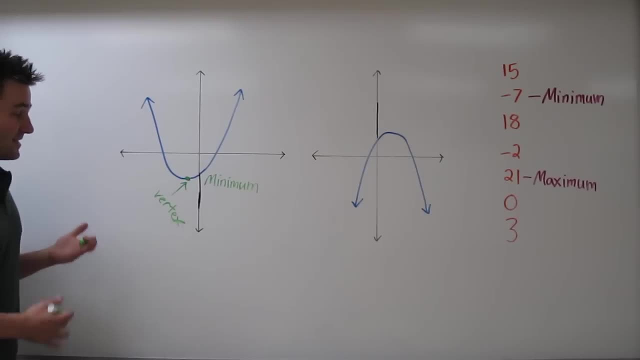 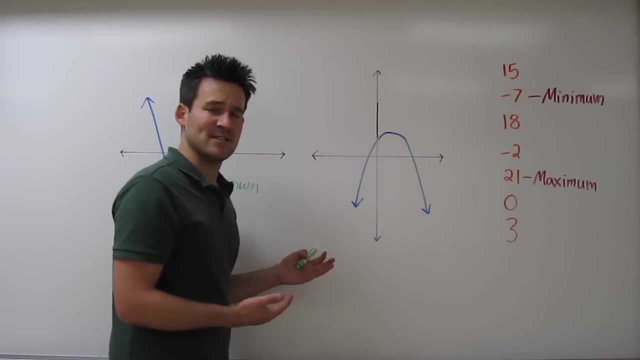 So on this parabola, the vertex is where the minimum value of the function is. Now let's look at this one. On this one we have a different situation. I can see that this right up here is the maximum value of the function. 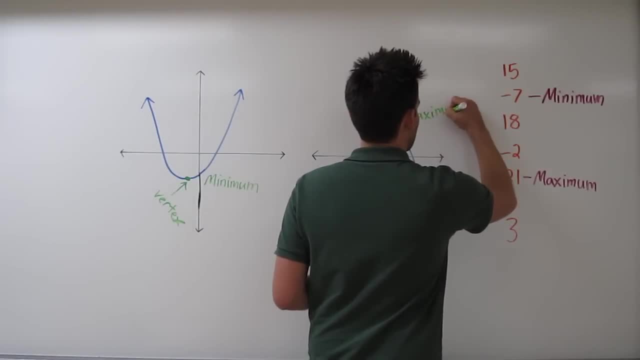 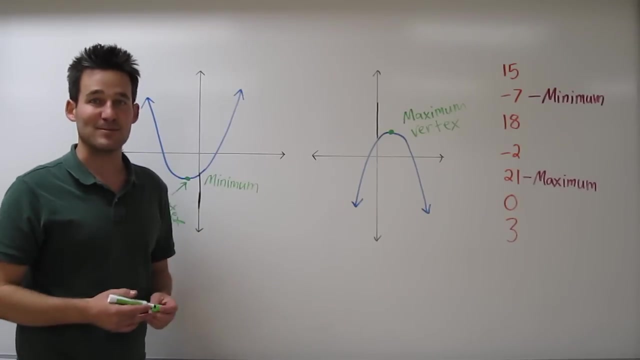 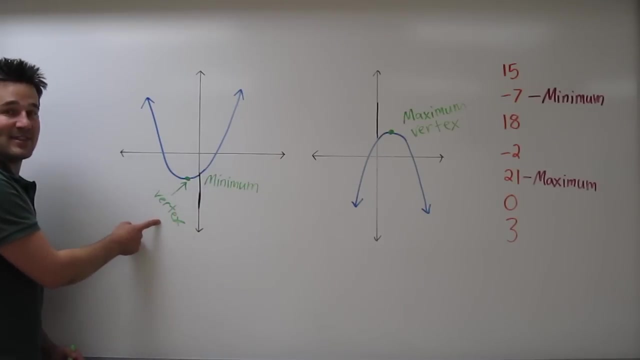 So I'll write maximum. And again, the maximum is located at the vertex. We can't identify a minimum value because those arrows indicate the function just keeps going down both here and here. What's interesting is that the minimum value was at the vertex on this parabola. 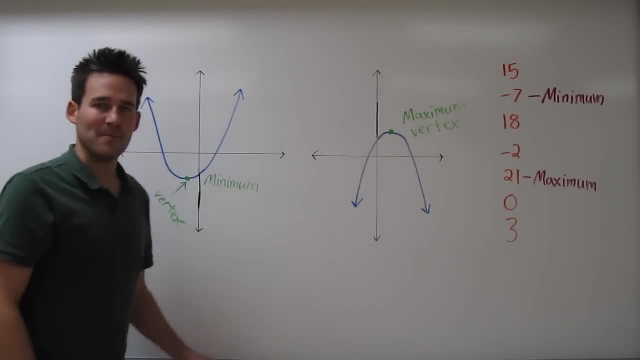 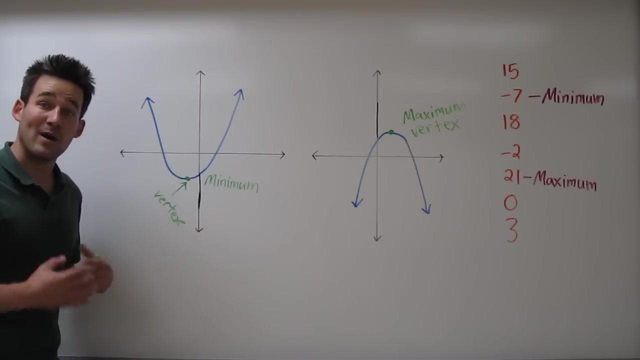 And over here the maximum value was on the vertex. here Now I say minimum and maximum and I'm saying value too. Well, if we were going to try to find out what that actual value was instead of just pointing to it on the graph? 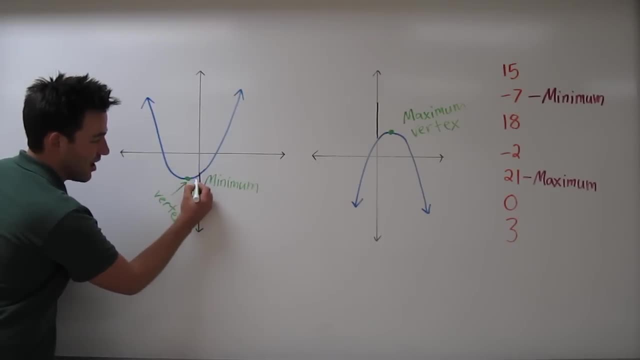 we would actually go to the vertex and draw a line over to the y-axis. Whatever value this is on the y-axis would actually be the minimum value Over here. whatever value this lined up with on the y-axis would actually be the maximum value. 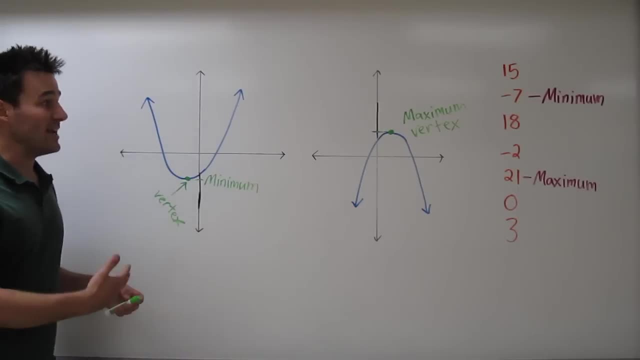 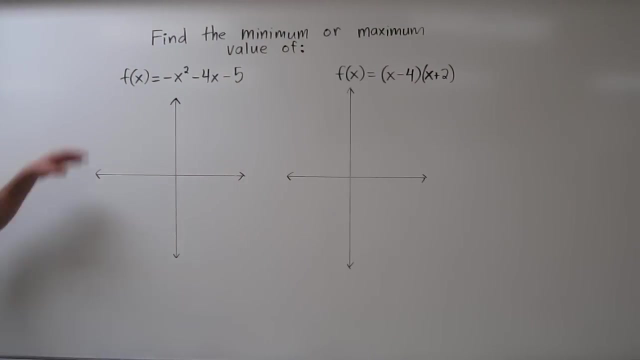 So let's try doing this with a few examples. Our instructions are to find the minimum or maximum value of two different parabolas. This first parabola is in standard form, That is, we have a function in ax squared plus bx plus c form. 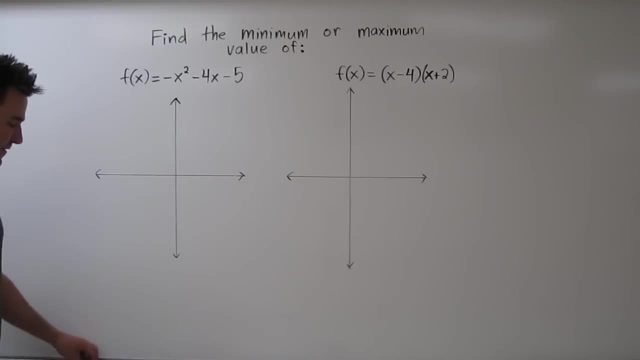 And if you remember standard form, we can find the vertex of the function by first finding what negative b over 2a is. That will give us the x coordinate of the vertex. So b, or the coefficient of the x term, is negative 4.. 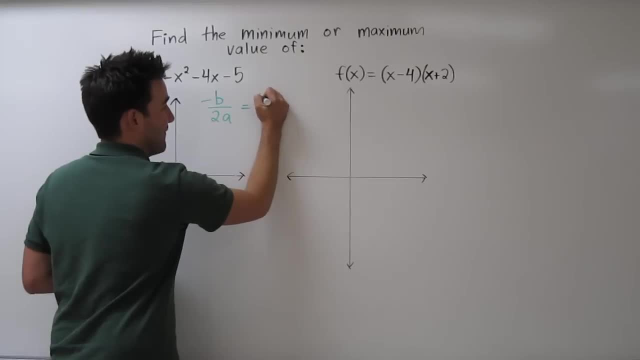 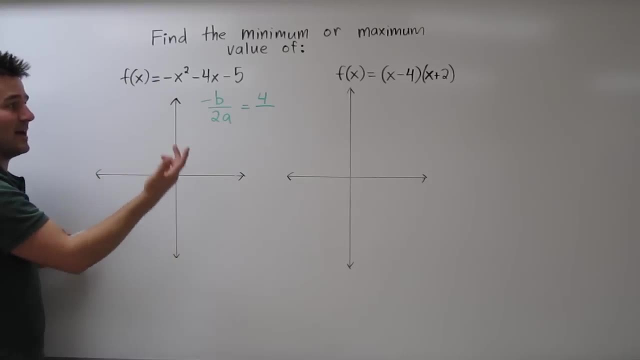 So negative, negative 4 is actually just 4.. And 2a: well, our a is negative 1, so 2 times negative, 1 is negative 2.. So it looks like we have when we reduce the x coordinate of the vertex is at negative 2.. 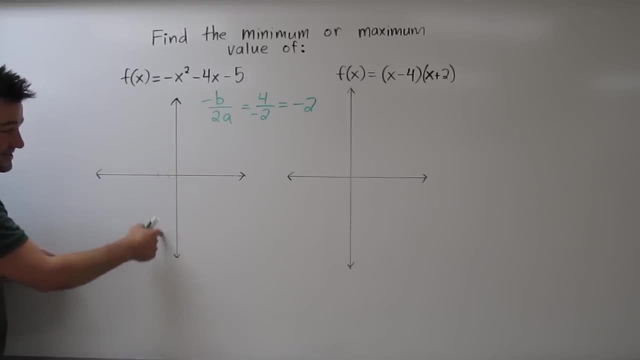 So let's see 1, 2.. The vertex is going to be somewhere at. the x is negative 2 line. Let's find out exactly where. To find that out, we're going to plug our negative 2 into the function. 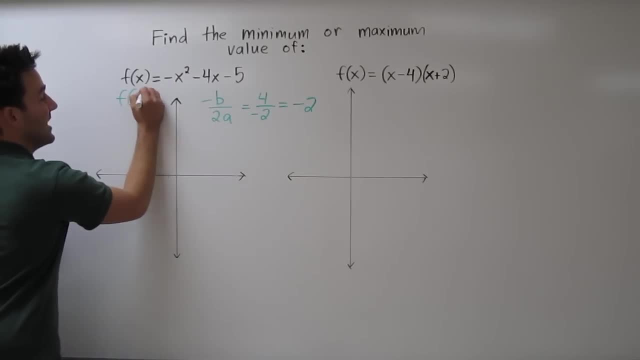 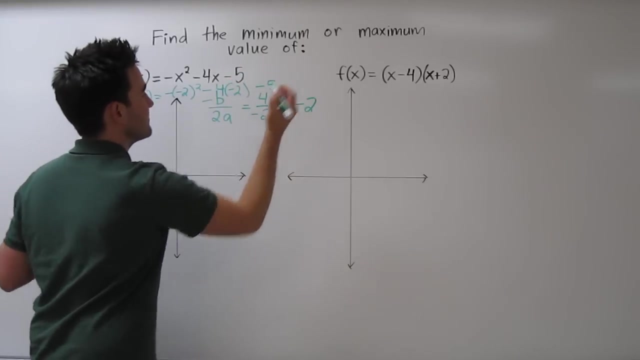 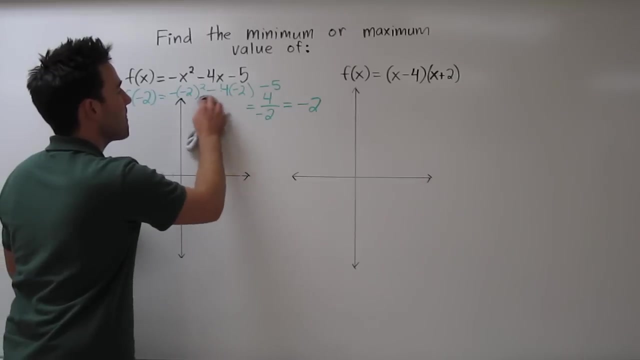 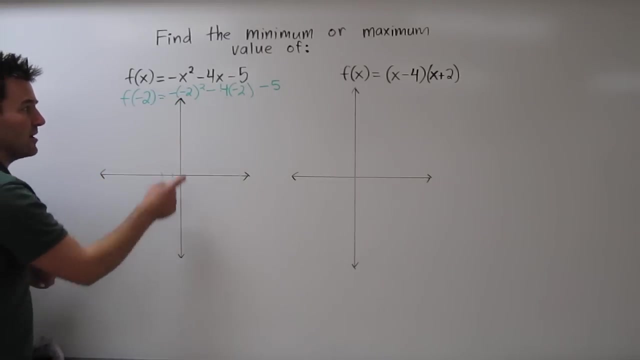 and we get. well, f of negative 2 is: let's plug a negative 2 in for the x squared there. I think we're going to kind of run out of room here. Let's erase a little bit. f of negative 2 is: well, negative 2 squared is 4 times negative, is negative 4,. 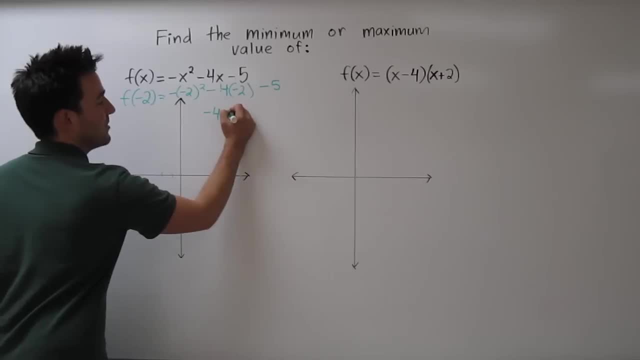 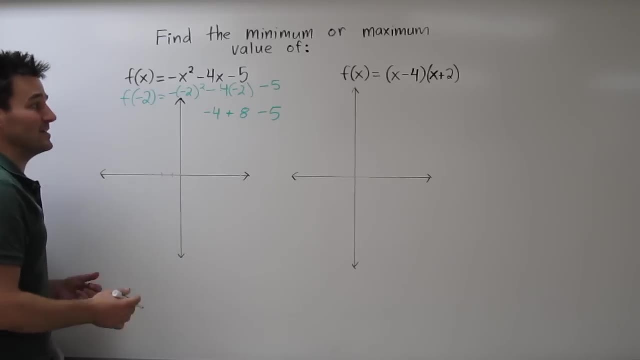 so we get negative 4 plus 8, minus 5.. Well, negative 4 plus 8 is 4, minus 5 brings us to negative 1. So that's our y coordinate of the vertex. So it looks like our vertex is going to be right there. 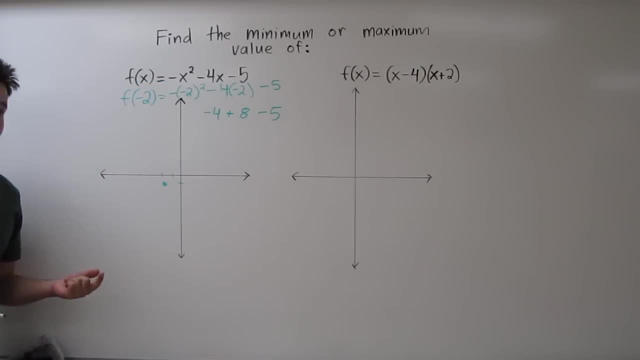 Also, by looking at the coefficient of the x squared term, we see that this parabola points down. So here's a rough graph of what this function looks like. Now, my goal was to find the minimum or maximum value of the function.